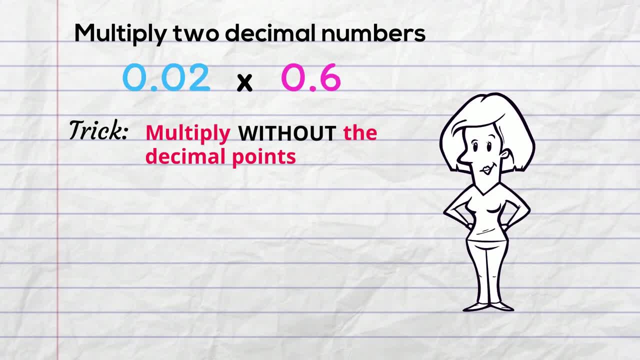 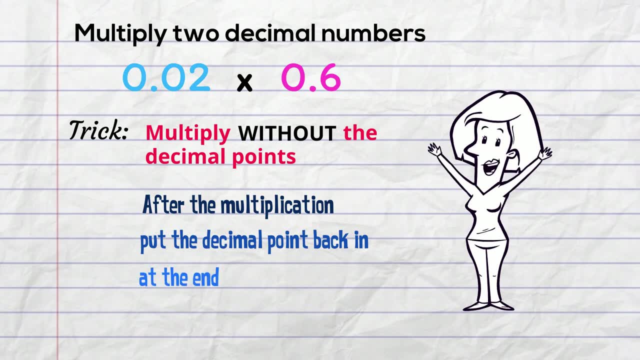 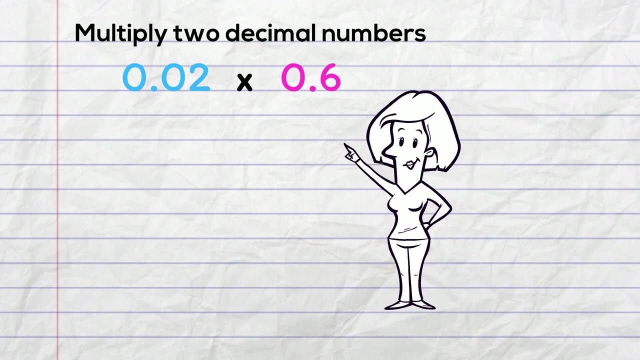 The trick is we multiply without thinking about the decimal points And then, after we've done the multiplication, we put the decimal point back in at the end, And that's where the counting part will come in. We start off thinking about these significant figures. 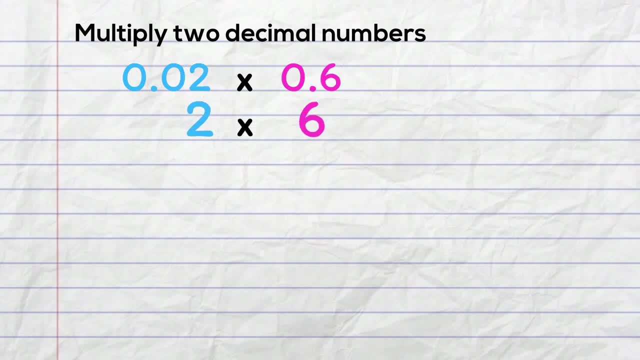 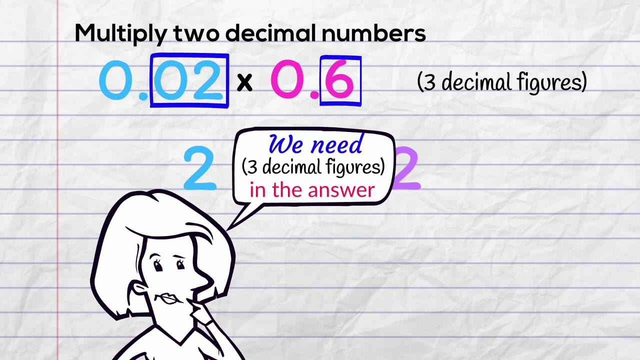 the 2 and the 6.. We multiply them together, Of course that's 12! And now we put those decimal places back into the answer. In the original we've got 2 decimal figures here and 1 here, And we need 3 decimal figures in the answer. 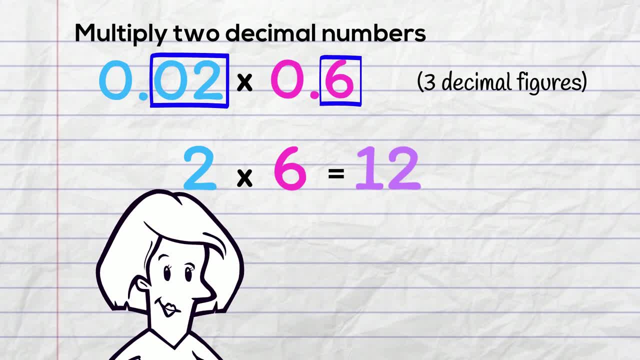 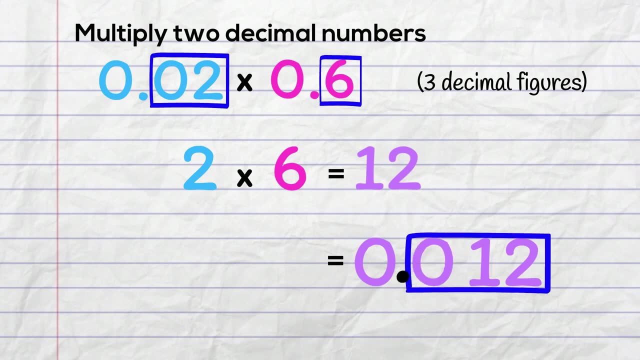 I only have 2 figures right now. Not a problem, I write a couple of zeros in front of my 12.. Starting from the right, we count to the left 1,, 2,, 3 figures, and here's the decimal point. 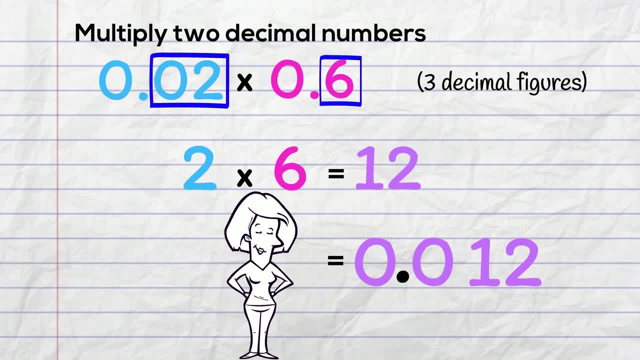 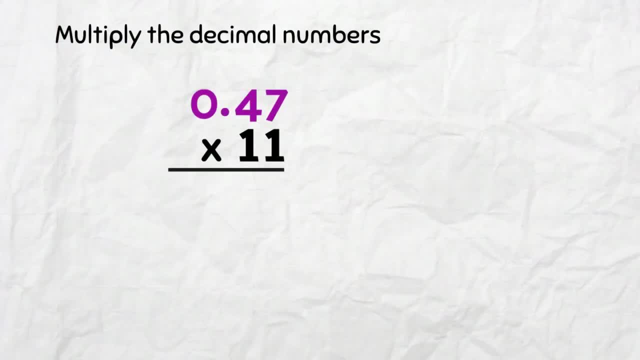 0.012.. I have 3 figures here, We're all done, And that's it. Let's do another one: 0.47 x 11, Ready to go in standard algorithm form. this time I'll ignore the decimal point right now. 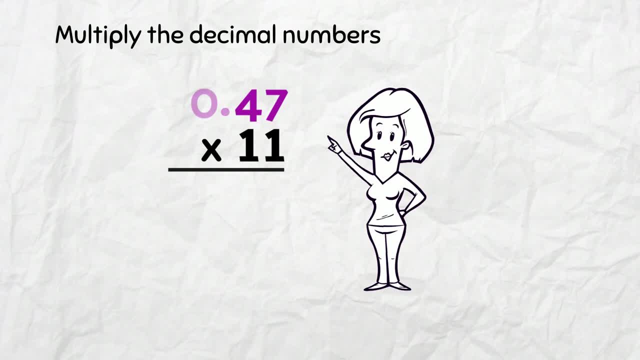 and just multiply like it's not even there. First row: 47 x 1, 47. Second row starts with a 0 because we're multiplying by 110.. 1 x 7 is 7 and 1 x 4 is 4.. 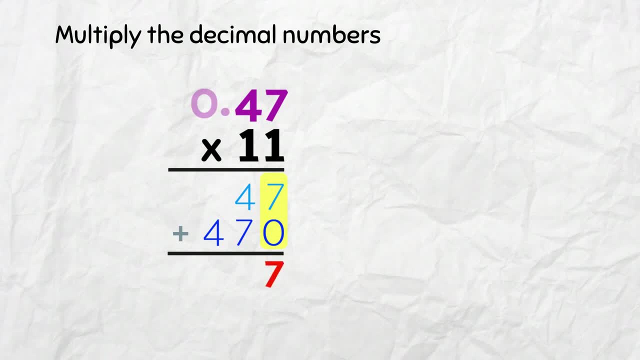 Now add them up: First row 7, Then 7 x 4 is 11, and here 4 x 1 is 5 517. Now we put in the decimal point. Here we have 2 decimal figures, So we need 2 decimal figures in the answer. 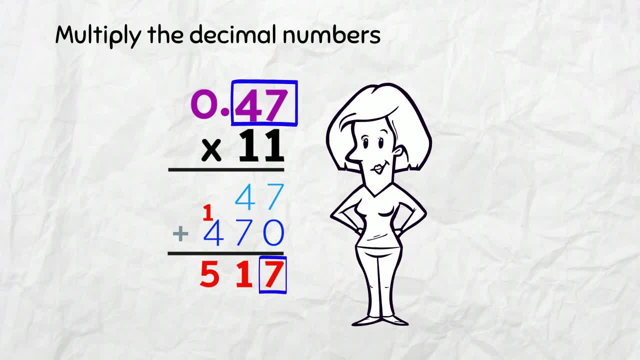 Count from the right to the left: 1, 2.. And there it is: 5.17- 2 decimal figures in the answer. All done, Pretty simple, right? Don't stop now, though, because there's a special case to watch out for. 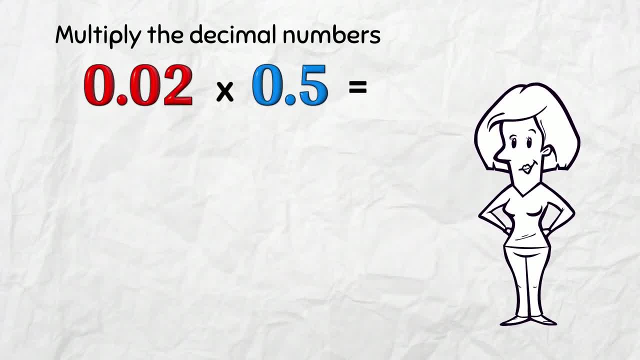 Like in this example, Always focus on the multiplication first. 2 x 5 is 10.. Notice it ends in a 0.. Ok, Now we put in the decimal figures- 2 figures here and 1 here, 3 decimal figures to go in the answer.